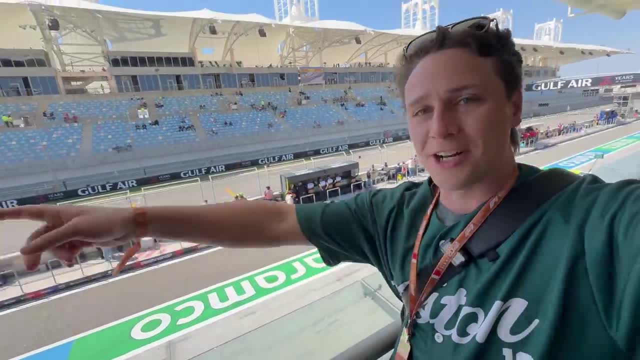 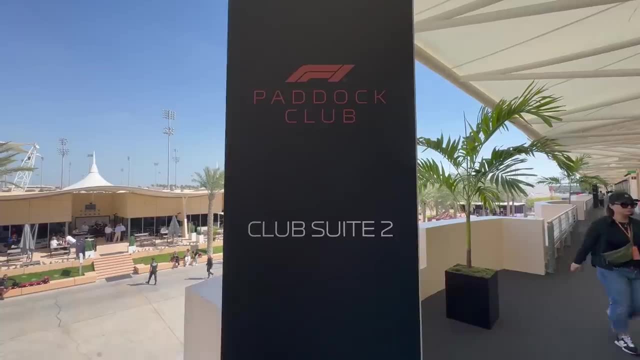 space. So you get to watch all the pit stops take place and the action, the start and the finish, right down the main street, And of course it has the champagne bar in the middle. Now, next to the lounge, is the paddock club suite with limited access. Not everyone is allowed in. 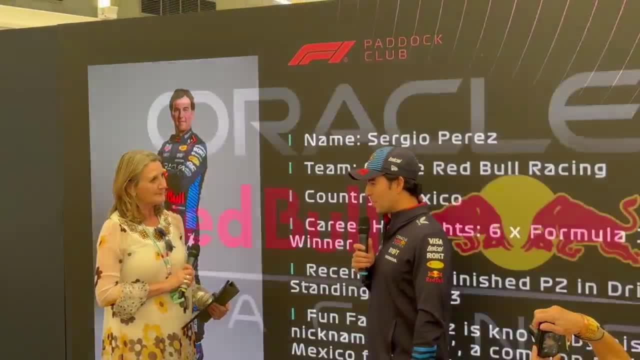 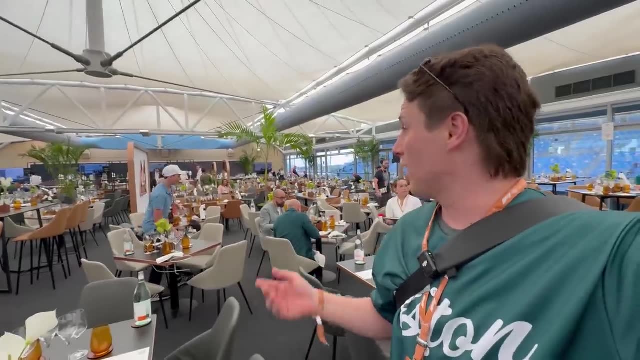 here. You never know who you'll meet in here. Wow, you can't get much closer than that, can you? While he's talking, I'll just show you the rest of the place. It's a real wine and dine type place. It's quite nice. It allows for sit down dining. Buffet stands around. 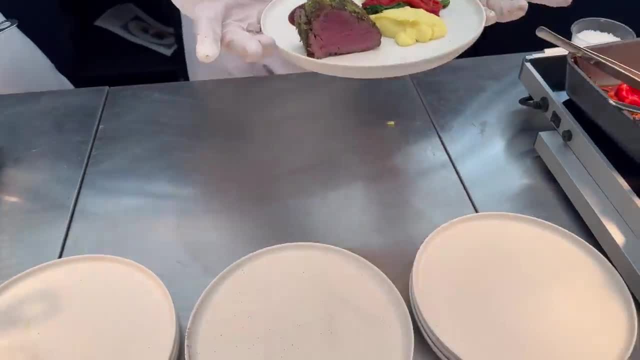 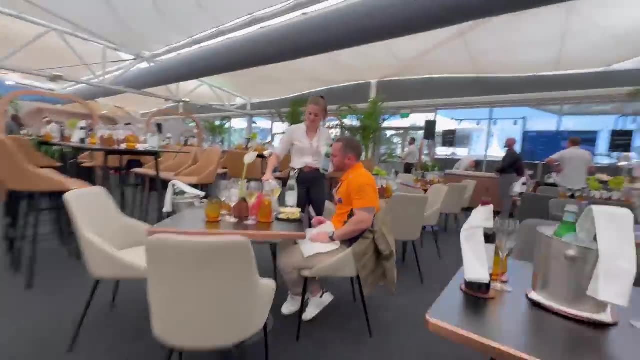 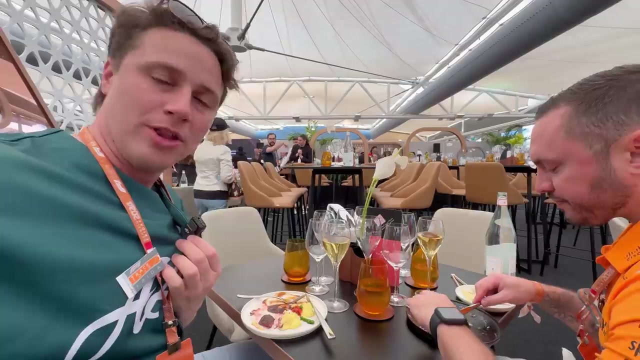 the edge with some incredible food. Wow, thank you. I mean, honestly, this is kind of like being in another world. This as the meal, amazing. This is like a shocking turning point in my life where the food and wine is so good That Ferrari driver Charles Leclerc is talking and I just 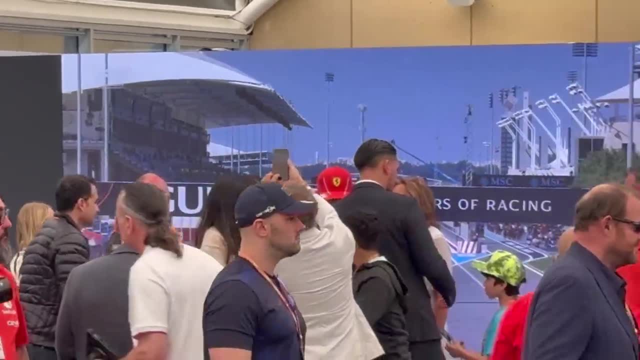 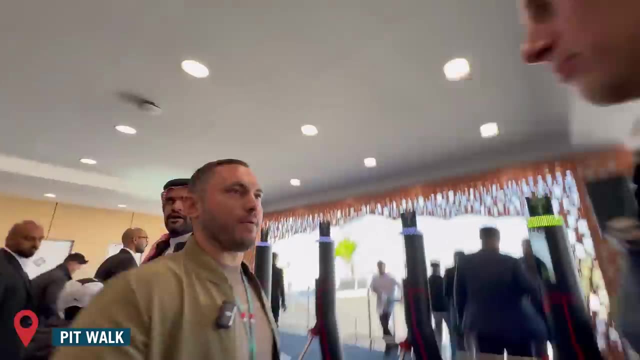 I'm focused. That doesn't mean we're not true fans. They just get absolutely bombarded by people. It's good to see them. Oh, what time does it? Right now, Okay, so we should do that now, Okay, okay, let's do that. 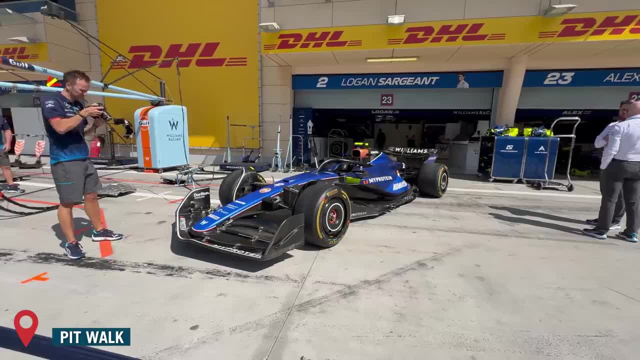 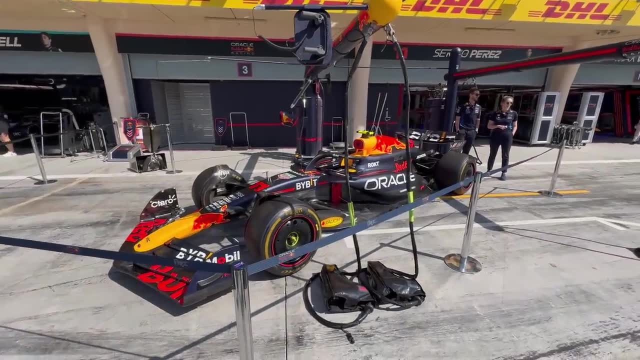 There are a couple of times on the race weekend where teams must put their vehicles outside for inspection. It's mandatory, Of course. at the end is the championship leader, Red Bull, down here, And well, they just happen to let some paddock club members roam around at this time too. 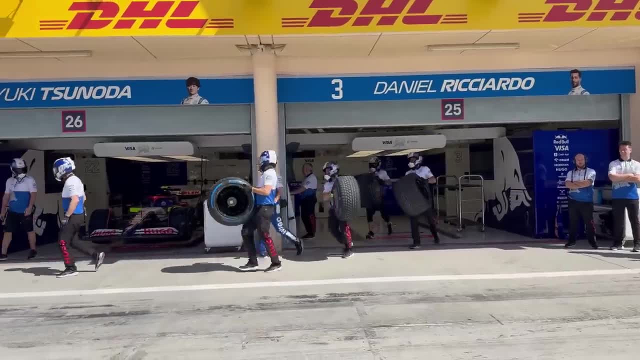 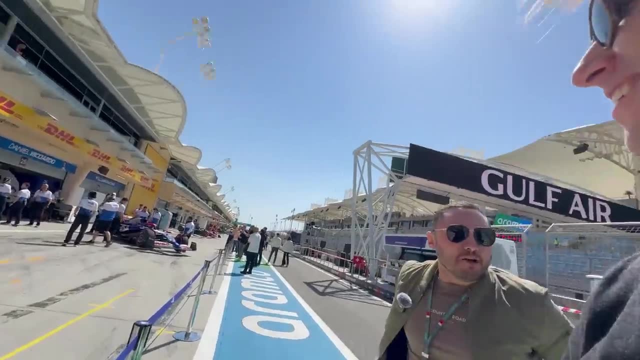 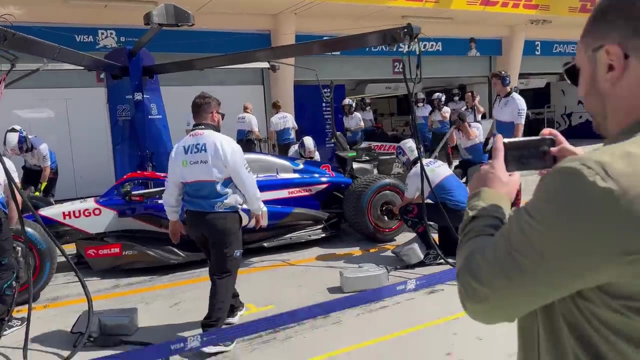 Oh, this is awesome, And some teams use this as an opportunity for a little practice as well. I think we're here right in time for Pitsbury. Let's stop practice. You're kidding? Wow, I am going to warn you. the noise is so loud it blew out my microphone, Jesus. 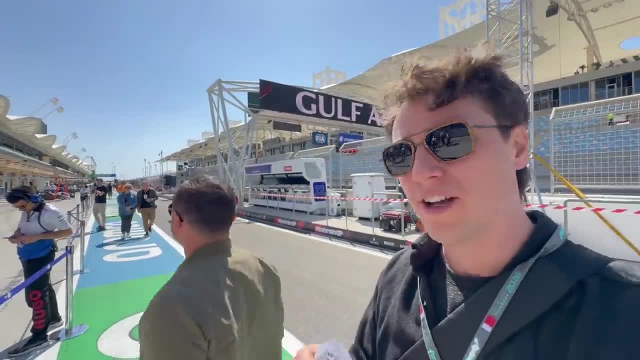 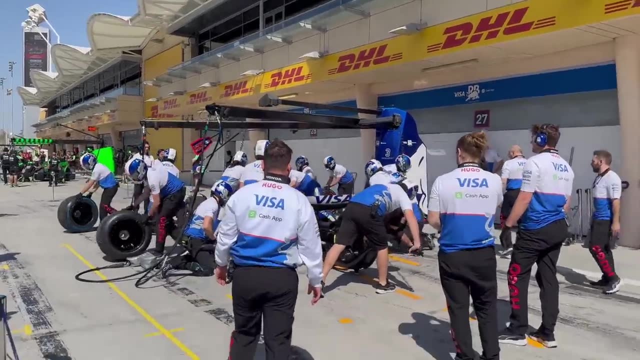 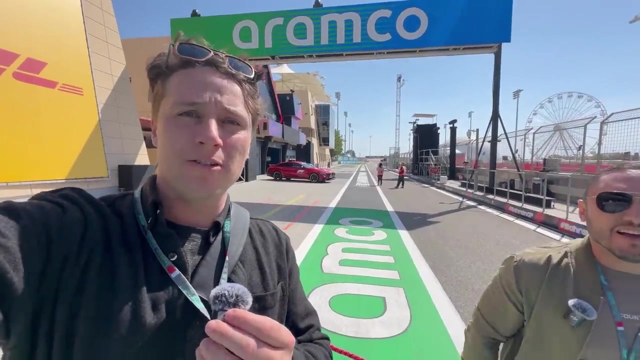 That's really loud in person. That is great. That is. the one difference of being here in person versus watching on TV is the sound and the feelings that you get. This is also our moment to see some of the drivers up close. There's Lance Stroll and Fernando Alonso. Now we've reached the end of the 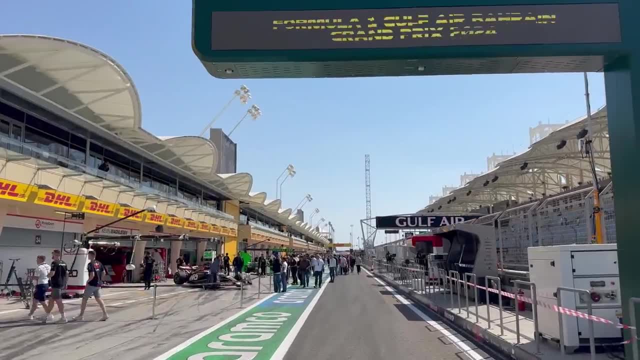 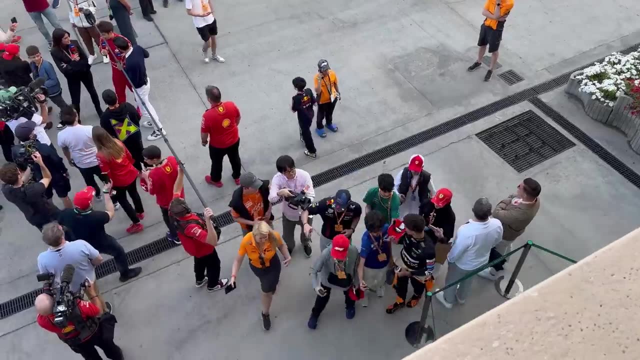 pit As a real F1 fan. amongst everything to do and see, maybe the best part is just leaning out over the balcony and watching drivers and media in the paddock. There's chaos. There's Lando, there's Charles Heck. I even spotted fellow YouTuber Kim Illman And, surprisingly, Gunther. 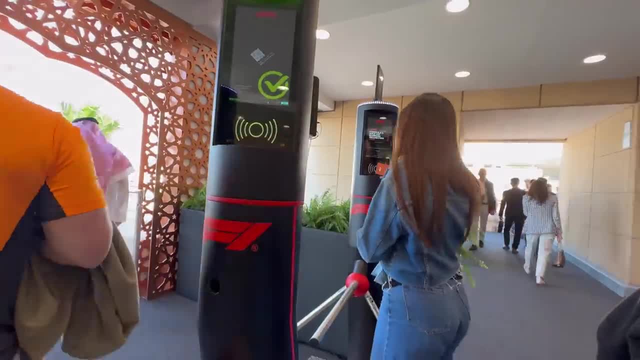 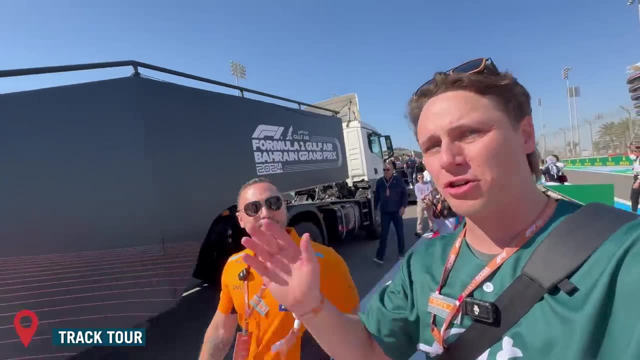 Steiner was here too. Next up, paddock club pass holders can sign up for a track tour. All right, we're going to the track tour. This feels like when the drivers do the driver's parade Feels a little bit like a Disneyland. They load us onto the back of special trucks. 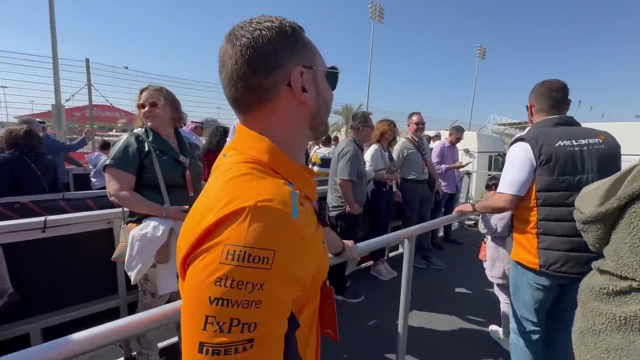 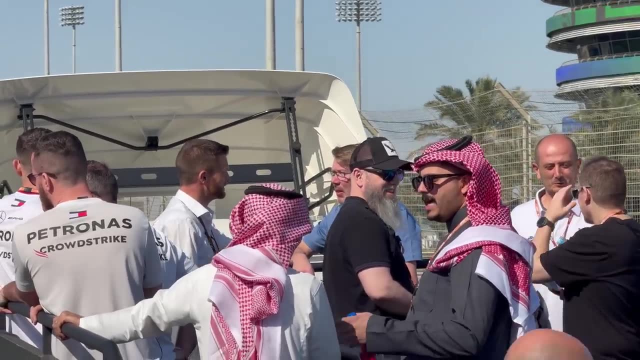 basically the same ones that they do the driver's parade on And they drive us around the track, starting on the main straight here. In fact, if you look closely, Mika Hakkinen was on the truck just next to us And off we go towards turn one. We're coming to turn one here, I mean. 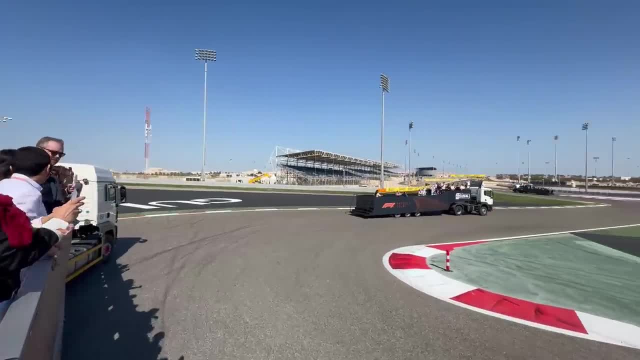 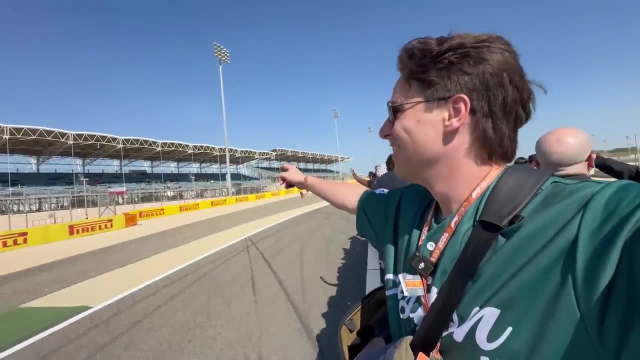 this corner is actually up into turn two and three. Turn one done And if you watched last year's video you'd know I was sitting right here. What you really notice on this track tour is just how long some of the straights are. I mean, obviously we're not going as fast as the F1 cars. 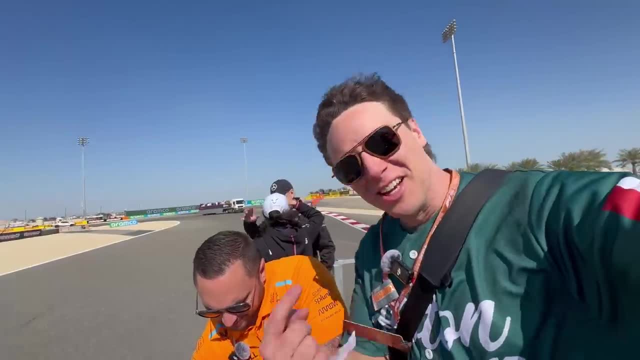 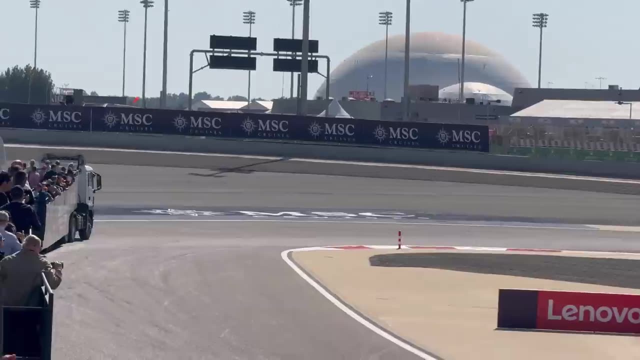 but you see this one, This is faster than I expected. You see my hair, We're moving. Yeah, We need to hear it. The other thing is just how tight some corners are. It's super interesting for all these guys out here. 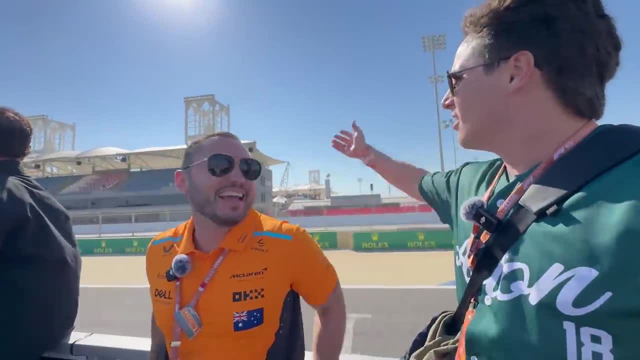 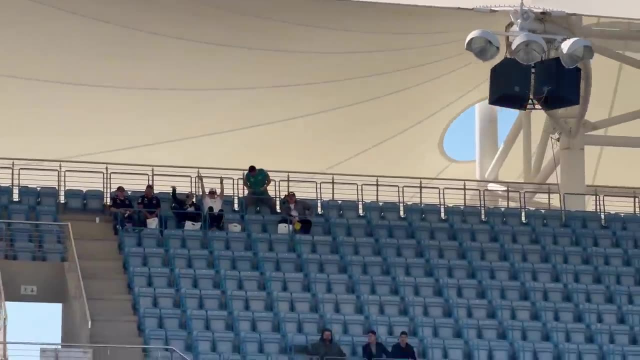 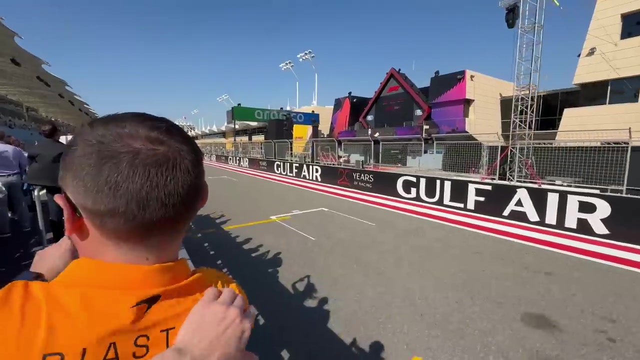 This is our driver parade moment. We'll never get another one like this. When you look outside, inside, did you notice how tight all the corners are? All in all, this was a very cool experience and it has me seeing the track differently. 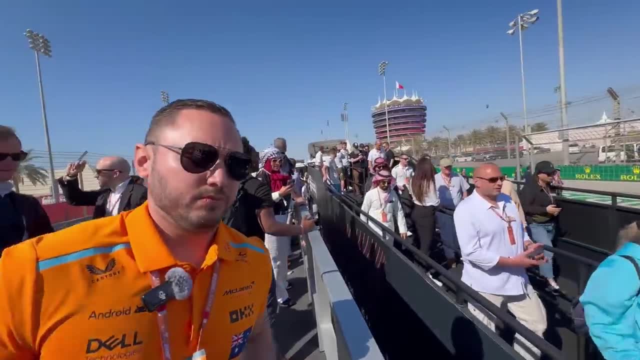 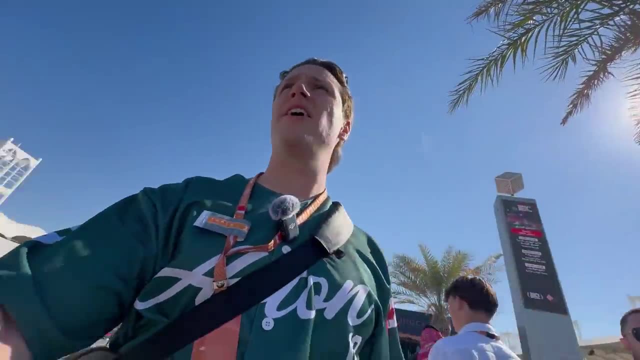 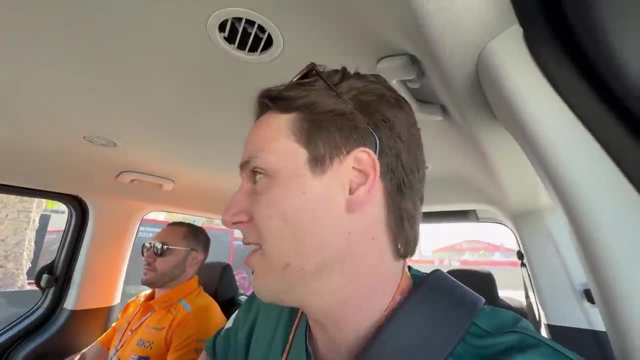 Actually speaking of seeing the track differently, there's one more place I want to show you. To get there, we're gonna need to take a special shuttle, only for Pata Club Pass holders. The Oasis Terrace is away from all of this action. It's kind of, as it sounds, an oasis in the middle of the track. 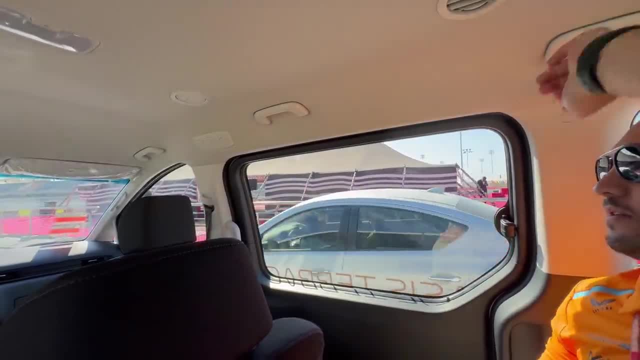 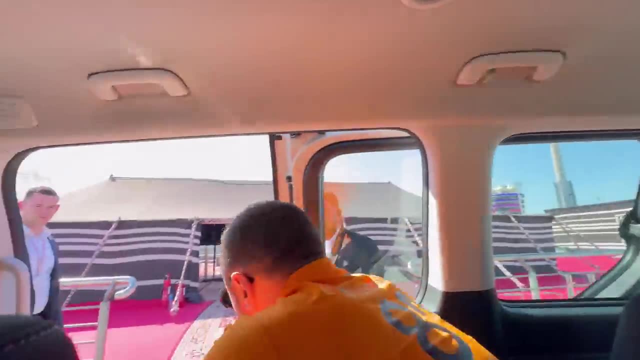 Because this is away from the paddock and the main straight. most people don't bother venturing out here, which means we have it almost all to ourselves, Thank you. So this is it: A little tent, a little oasis in the middle of the track, and we have on our right a little. 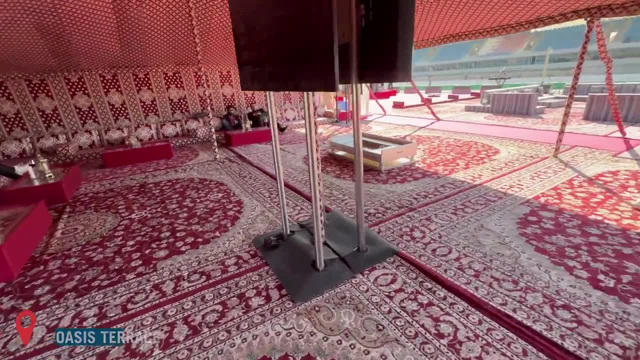 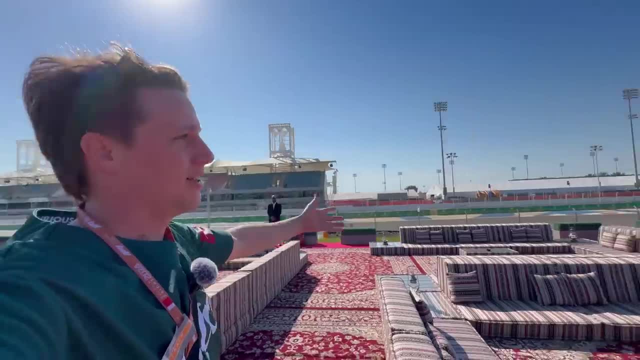 bar area, Buffet seating area on the left in the shade and, of course, you come out four seating areas out here with the back straight down here and the tower right there. There's not a lot of people that know about this place, but one spot in particular: that. 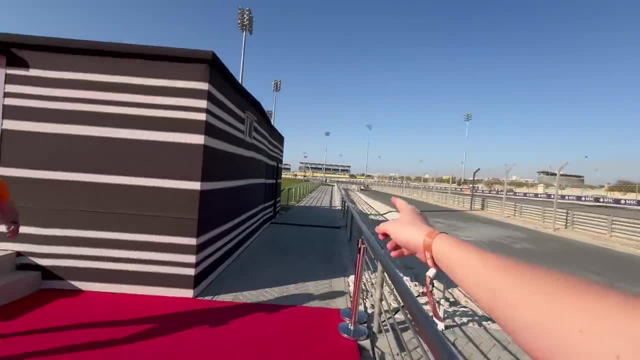 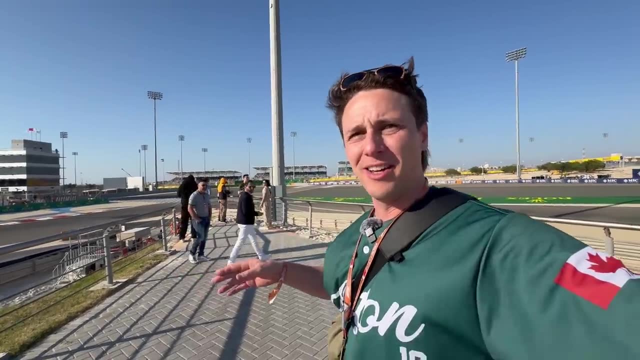 even fewer people know is just over there, so I'm gonna show you that Down here. So that walkway brings you out to this little platform here, which is right at the hairpin corner of Turn 11.. One of the things about being out here in Pata Club is you never know who's gonna be. 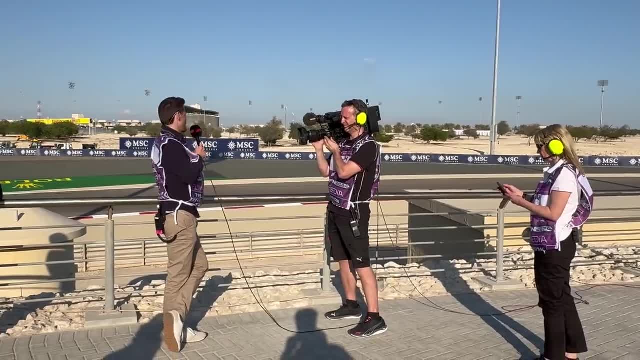 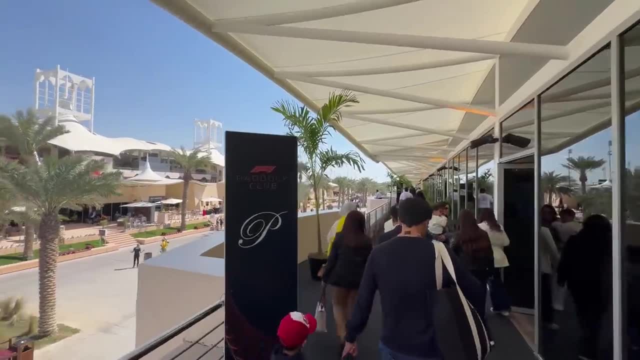 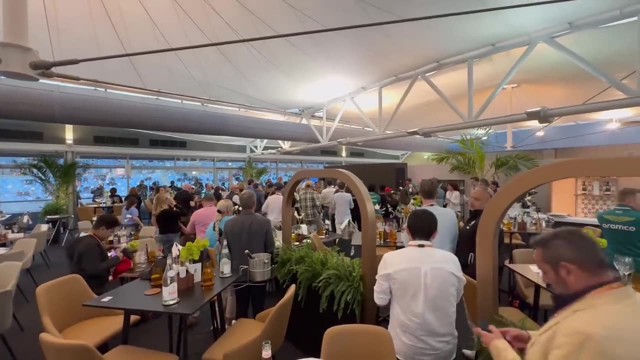 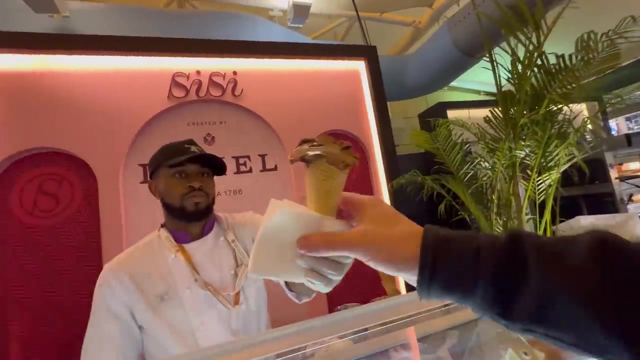 around. We've decided to go back to the Pata Club to get some dinner, when it was all pleasantly interrupted by Fernando Alonso of all people. But the evening is getting darker, which means the race is about to happen. so it's time for a little dessert and get settled in for some more celebrity spotting. 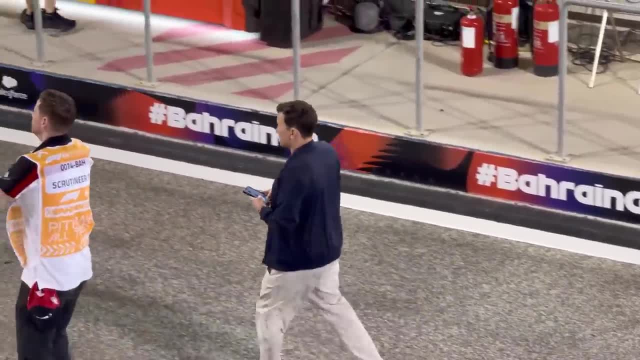 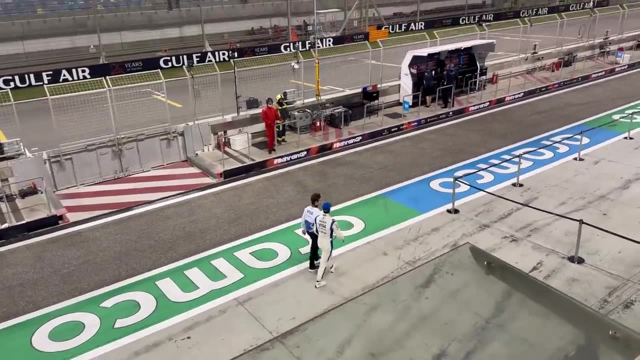 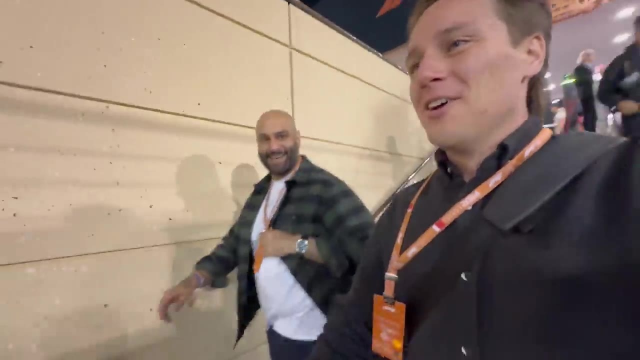 Ozzy legend. Ozzy, great baby. I mean, really, It's the first race of the season. Everybody is here, Ozzy, Ozzy, Ozzy. It's Oscar Piastri, Not yet a world champion. Now, at this point, Ammar, here, a new friend and local Bahraini, wants to take me back. 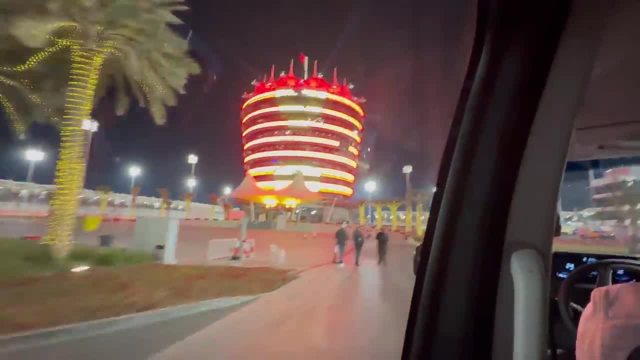 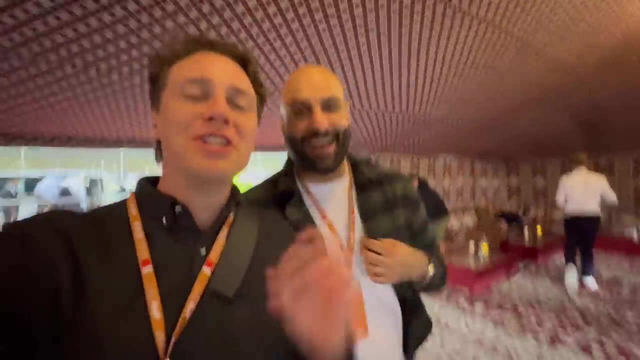 to the Oasis Terrace to show me a local tradition. Thank you, Nice place. How do you describe this place? This is Bedouin. This is gonna be so good. Bedouin chic, Bedouin chic. I love that. 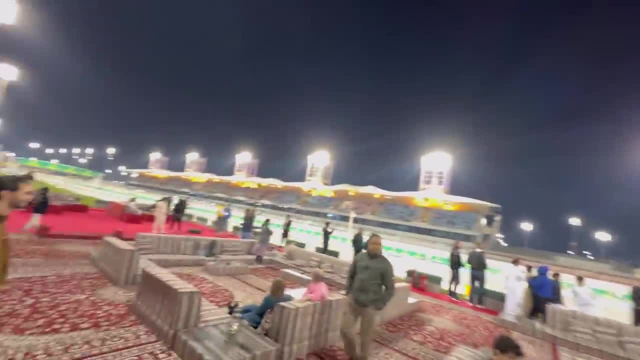 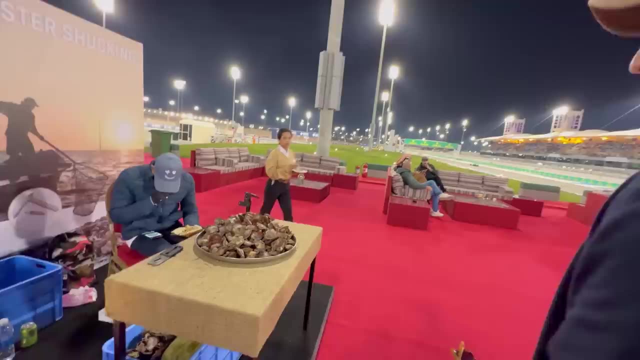 Wow, And this place looks even better at night. Wow, Wow, This is Pata Club elevated. You might get lucky. Yeah, You might get a nice Bahraini pearl. Oh a pearl. You're known for pearls. Wait, wait. 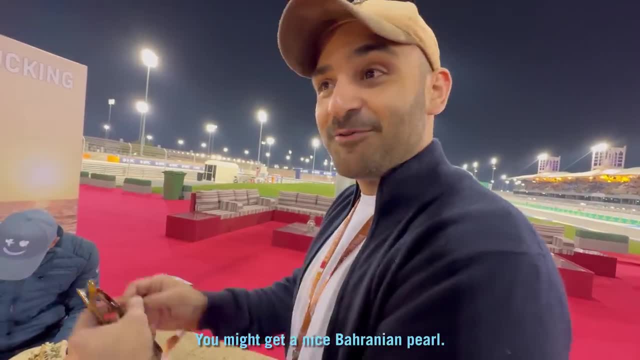 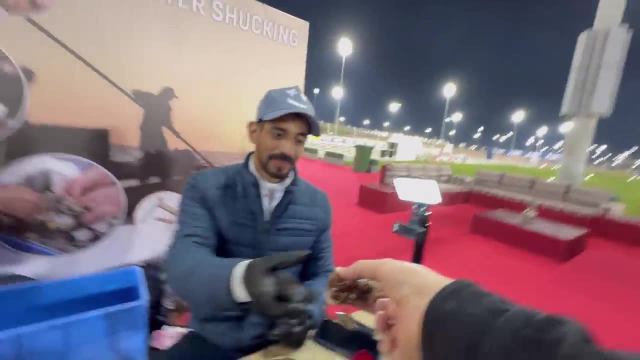 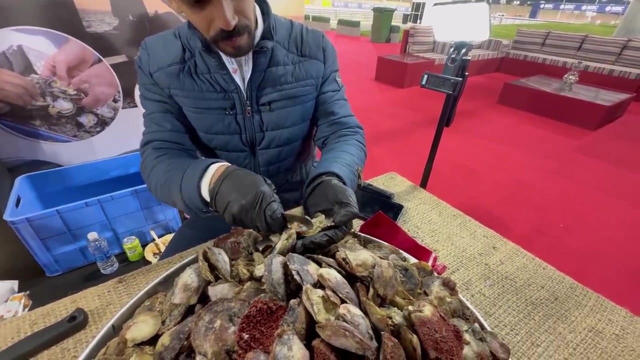 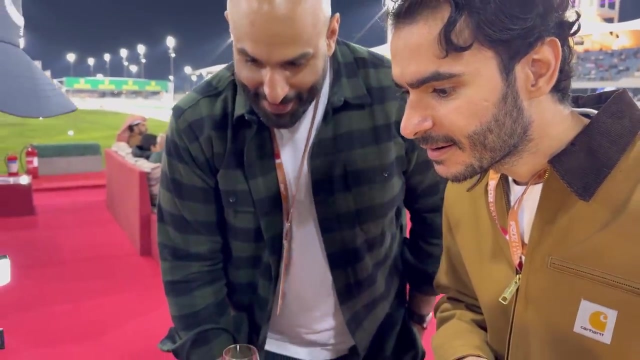 I want this one. You see, Bahrain is a small island country that traditionally fished oysters to find pearls, And it's a tradition that they keep today. The question is: will I get lucky? Is that a pearl? That's a pearl.